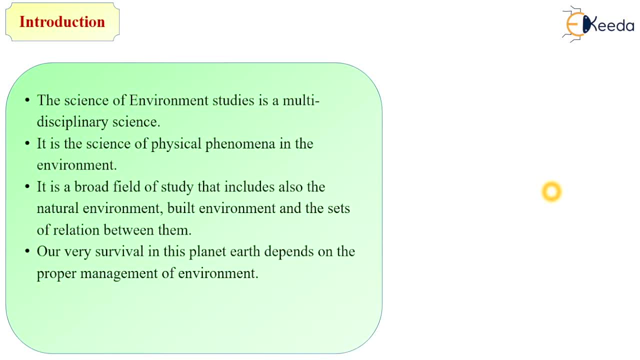 Our survival in this planet earth depend on the proper management of environment. Every living being are interdependent directly or indirectly. That means environmental management is a part of environment or a science of environment, in which we are studying the physical phenomena of environment as well as the broad field of study that includes the natural environment, built environment and the set of relation between the natural and built environment. 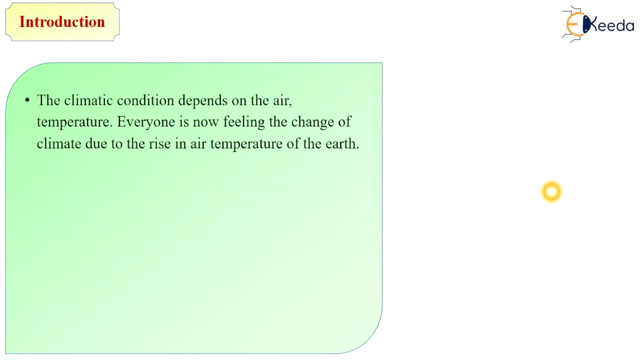 Also, while studying the environmental management system, We are also studying the existence of natural resources, of the climatic conditions, which are depends on the air and temperature. Everyone is now feeling the change of climate due to the rise in air temperature of earth, More presence of carbon dioxide is resulting ozone layer. 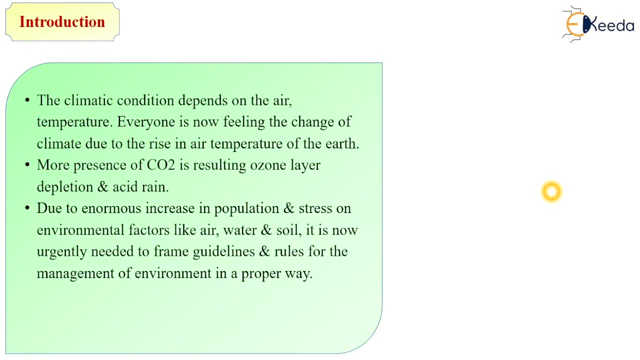 depletion and acid rain, and due to enormous increase in population and stress on environmental factors like air, water and soil, it is now urgently needed to frame guidelines and rules for the management of environment in a proper way. A good management of environment can only bring a sustainable life to all in. 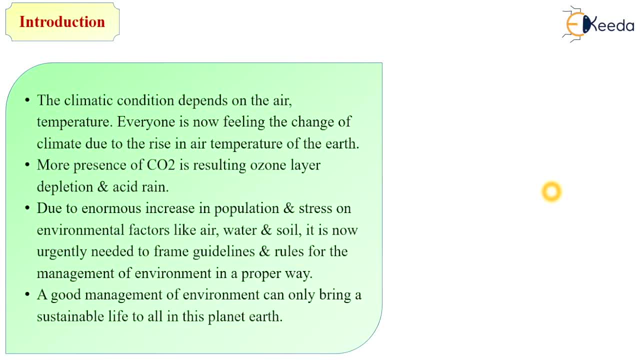 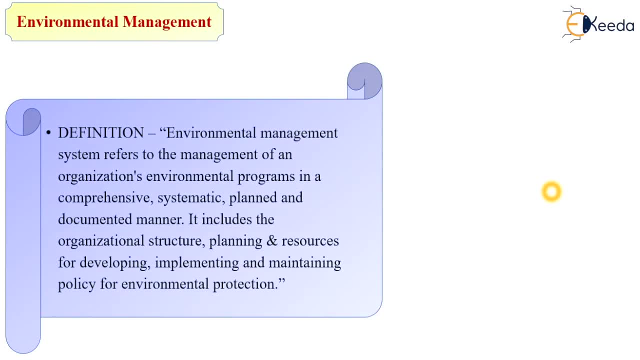 this planet earth. So now we are exactly learn the what is environmental management? So environmental management system refers to the management of an organization's environmental programs in a comprehensive, systematic, plan and documented manner. It includes the organizational structure, planning resources for developing, implementing and maintaining policies for. 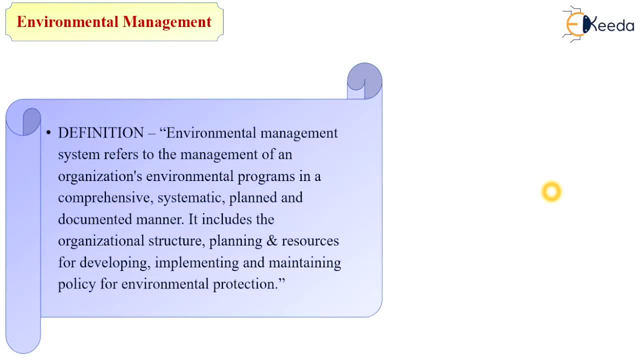 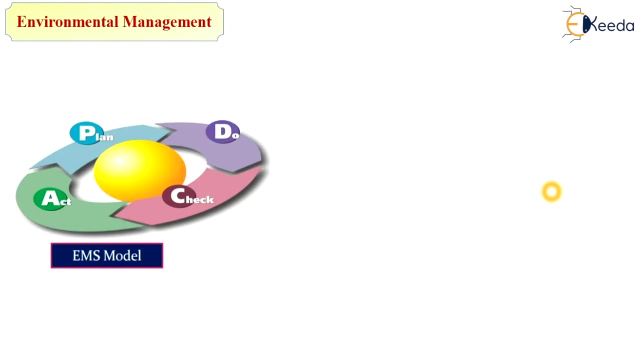 environmental protection. So it is necessary to protect our environment and for that we are providing a a management, environmental management system which includes the systematic plan and document documentation of all the things. so, as you can see in this diagram, so environmental management, or the principle of environmental management, includes the plan, do check and action. so which? 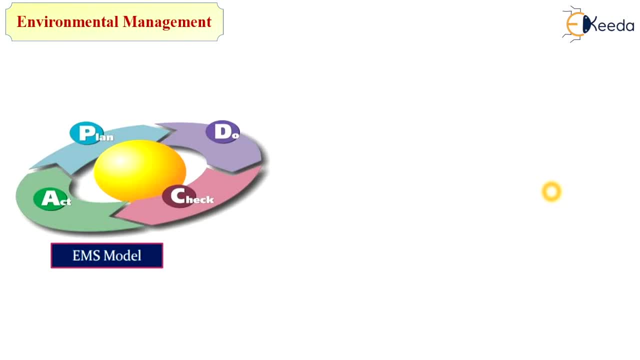 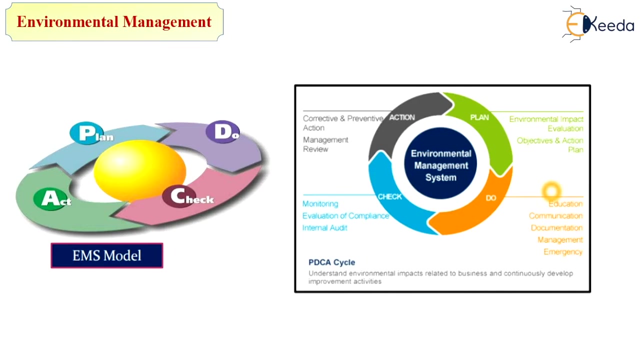 is based on. the environmental management system is based on this four principle, that is, plan, do, shake and action or act. so let's we see the. what is that mean? or what we are doing in plan, what we are doing in do principle, what we are doing in shake principle and what we are doing in action. 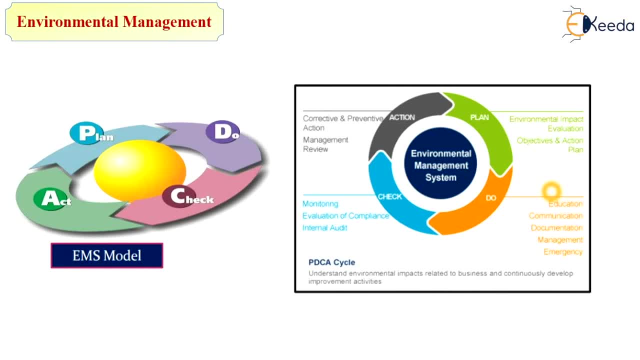 principle. so let's we see one by one principle. so first is plan. so it is the first step in environmental management system. so in planning we are set some objectives and action plans depending on our ultimate goal. so it is the first step of setting the standards in environmental. 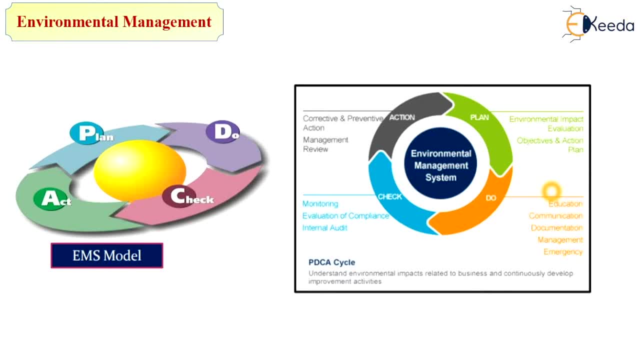 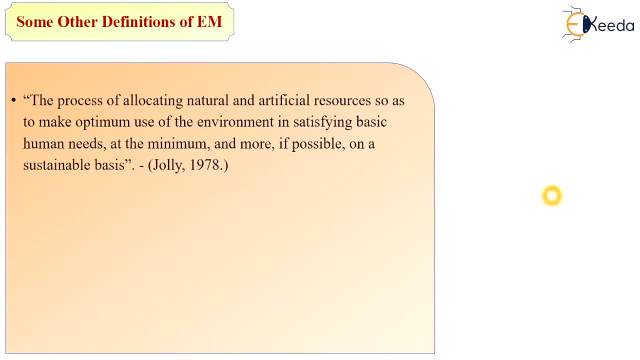 management system. that is plan, and in planning we have set objectives and action plan. definitions of environmental managements are: it is the process of allocating natural and artificial resources so as to make optimum use of environment in a satisfying basis: human need at the minimum and more, if possible, on a sustainable basis. 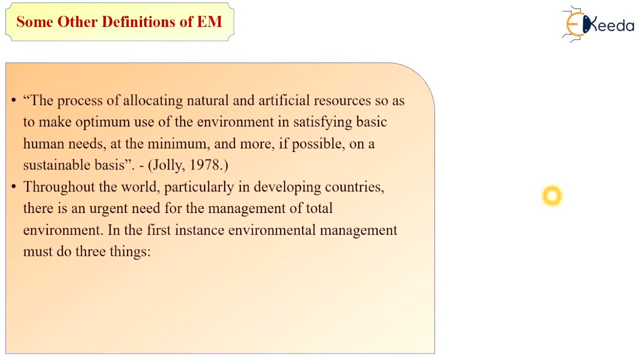 again. in other words, particularly in developing countries, there is an urgent need for a management of total environment. in the first instance, environmental management must do three things: first is identify the goals. second is establishing whether this can be met or not. and third is develop and implement means to do what it deems possible. that we have seen in principles of 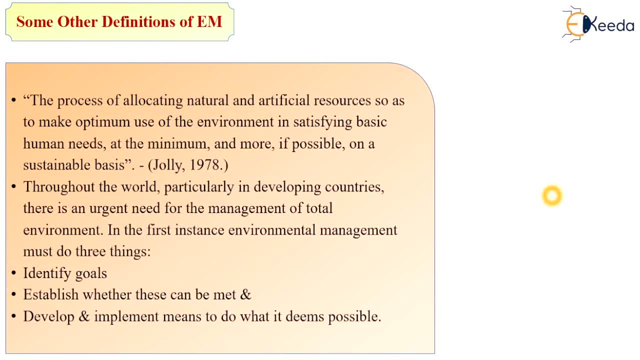 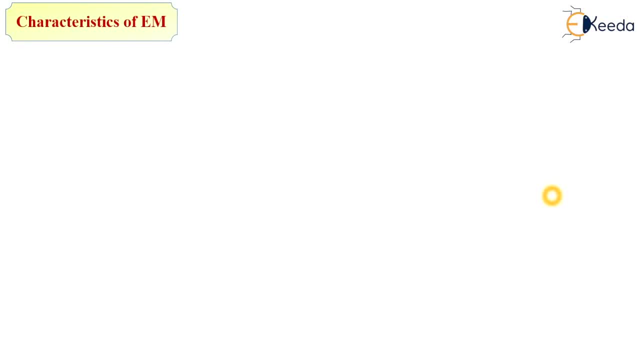 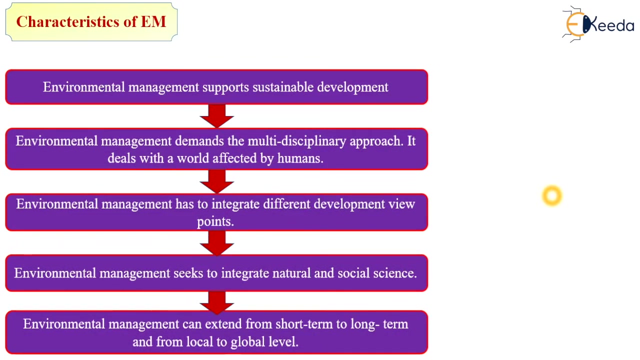 environmental management system that are the plan, do check and action. so these are some definitions in different words of environmental management system, so you can use any one of these definitions. so next are the characteristics of environmental management. as you can see in flowchart, these are the characteristics of environmental management. 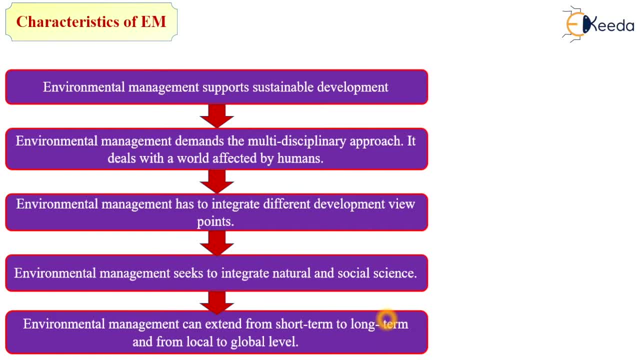 first is: environmental management supports sustainable development. it is very important point. so we are following the environmental management system. that means we are doing the practice of sustainable development of environment. second characteristics is environmental management. management demands the multidisciplinary approach. it deals with a world affected by humans. 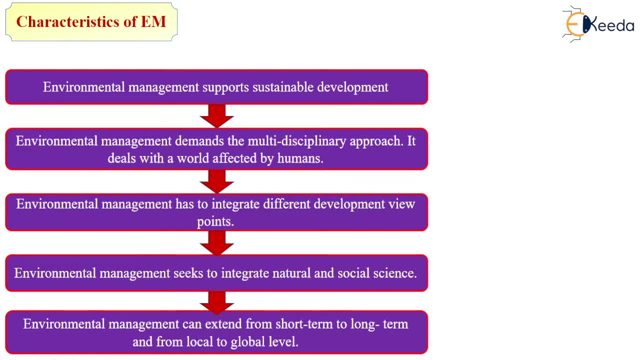 third characteristics is environmental management has to integrate different development views. point. next characteristics is: environmental management seeks to integrate natural and social science, so it is the combination of natural as well as social science. and last one is environmental management can extend from short term to long term goals and from local to global level. so these are: 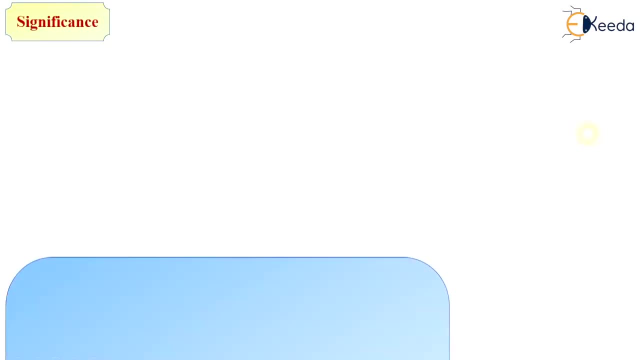 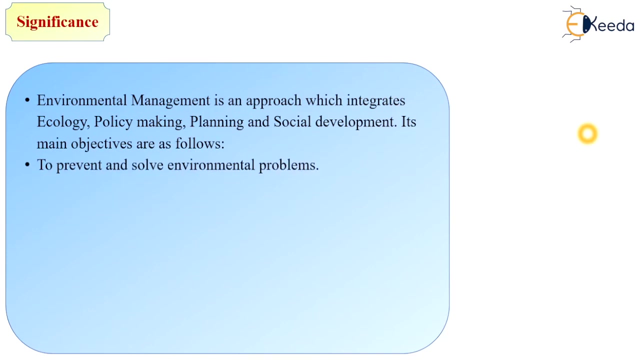 the characteristics of environmental management system. next is: what are the significance of environmental management? Environmental management is an approach which integrates ecology, policy-making, planning and social development. Its main objectives are as follows. First is to prevent and solve environmental problem. To establish limits in terms of some permissible limit or discharge standards. 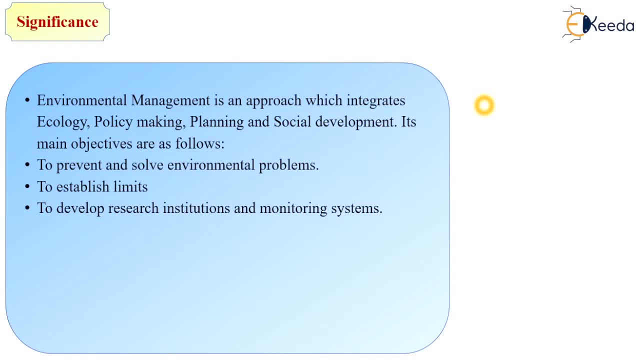 Next, to develop research institutions and monitoring systems. Next, to warn threat and identify opportunities. Next, to suggest major for resources conservation. Next, to develop a strategy for a improvement of quality of environment. and to suggest long-term and short-term policies for sustainable development. 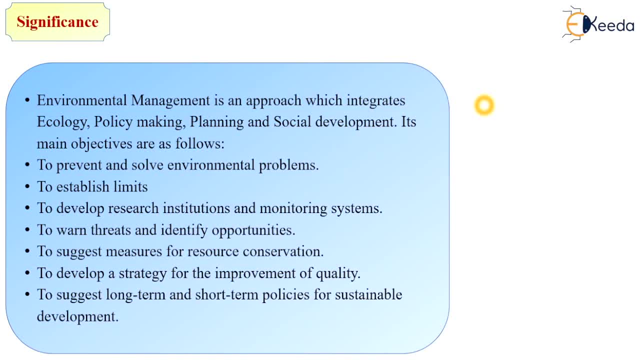 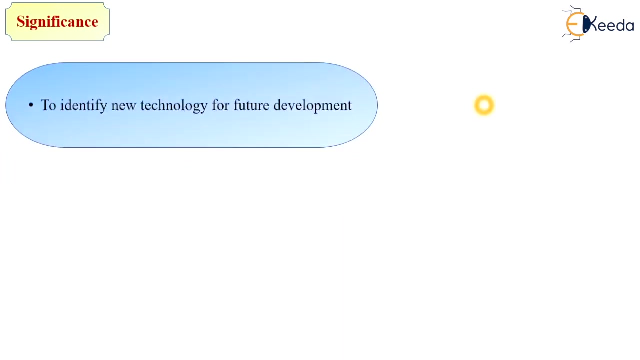 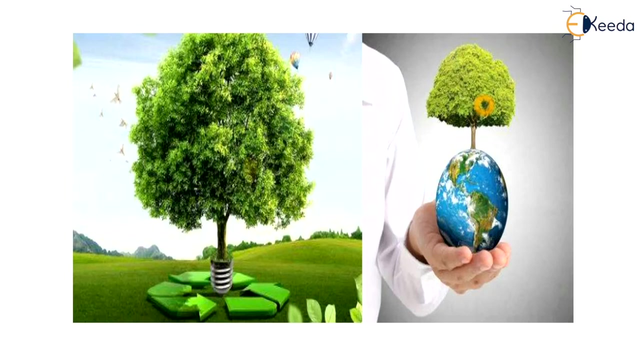 So these are the significance of environmentalism And it is very important to follow the plan or actions related to environmental management system or to use the environmental management policies. And the last significance is to identify new technology for future development. So to study the environmental management system.